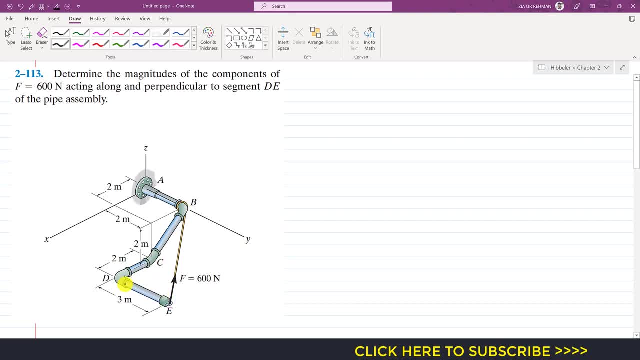 the components of this force F along this DE and perpendicular to this DE pipe. So we need to find the Cartesian vector representation of this force F. And so the Cartesian vector representation of force F is, we know that it will be equal to its magnitude times the. 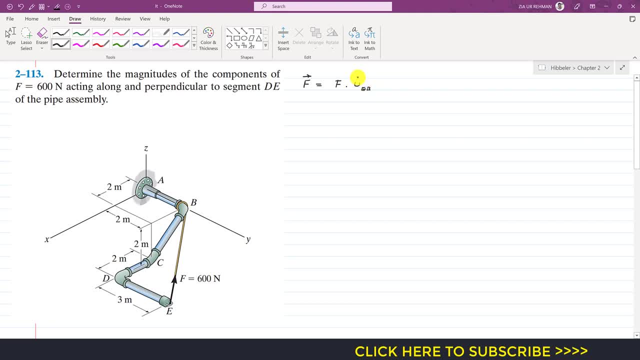 unit vector from E to B, since the force is acting from E to B And the magnitude of the force is given, which is 600.. So I will write 600 multiplied by the unit vector from E to B, then this will be equal to 600. And then we can find the unit vector from E to B by: 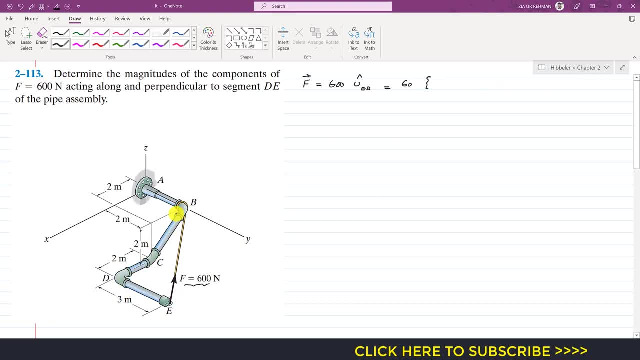 moving from E along the x, y and z axis until we reach that point B. So to reach that point B we need to move two meters. plus this two meters distance in the negative x direction. right, So I will write 4i In the negative i. we need to move two plus two, four meters distance in the negative. 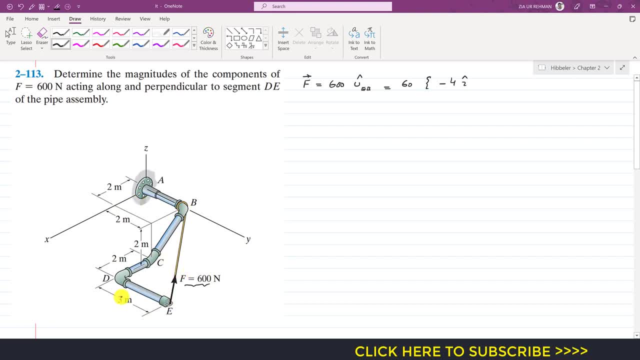 i direction, In the negative j direction, we need to move three meters distance right. So we need to move. in the negative y, we need to move three meters distance. So I will write minus 3j. And from E to B in the z direction, we need to move two meters distance and that 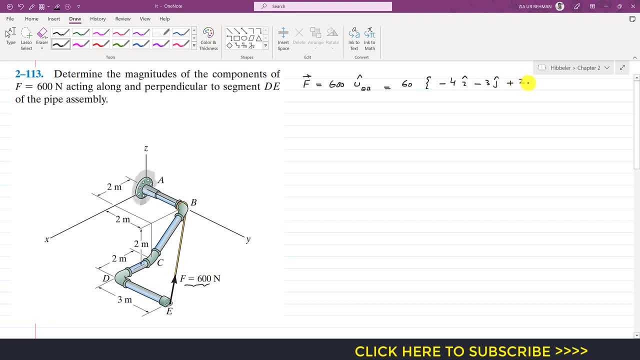 is in the positive z direction, So this means that we need to move two meters distance in the positive k direction. So this is the position vector from E to B, Since the unit vector from E to B is equal to the position vector from E to B divided by the 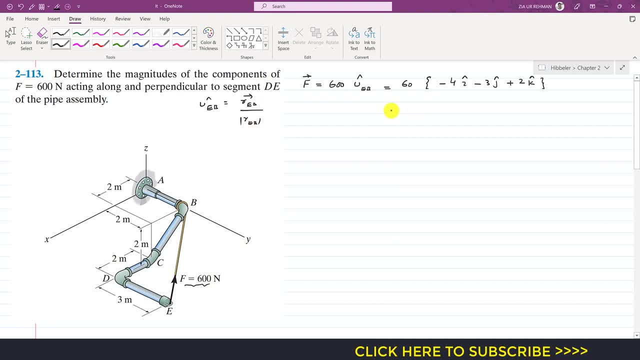 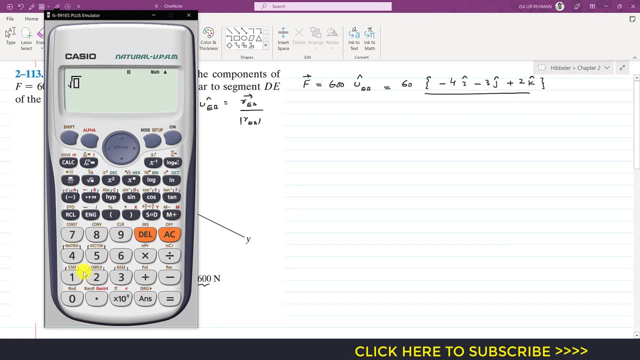 magnitude of the position vector from E to B. So this we can find the magnitude of this position vector, so I will do it directly in calculator. So this will be equal to four squared 5.. jeżeli 4a разu, 5dmizeZm i, 4hq3 M MediaWanRT X v E, 2m6 dessa, VANmNus Nm vRs 0,dB, zAVZnBZ, 7OZZn0ZZuYZiZZl, engRas harline R,0. 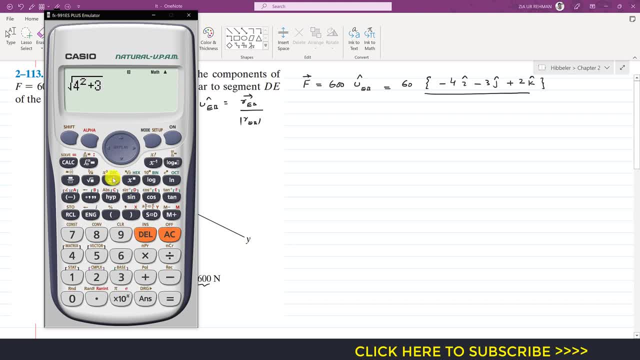 will take the squares of the magnitudes of the components. so this is 4 square plus 3 square plus 2 square, and then we will take the square root. so square root 29 is the magnitude of that position vector from e to b. so this is 5.385, so 5.385, so this is the magnitude. and now 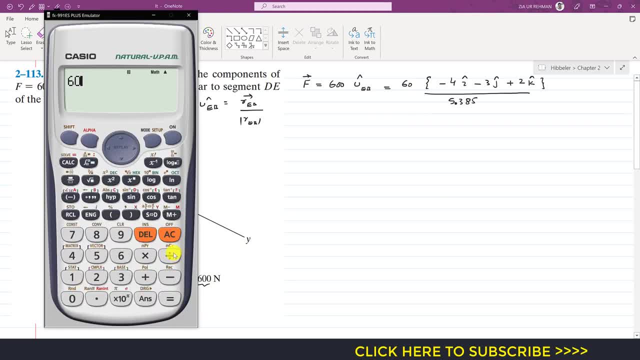 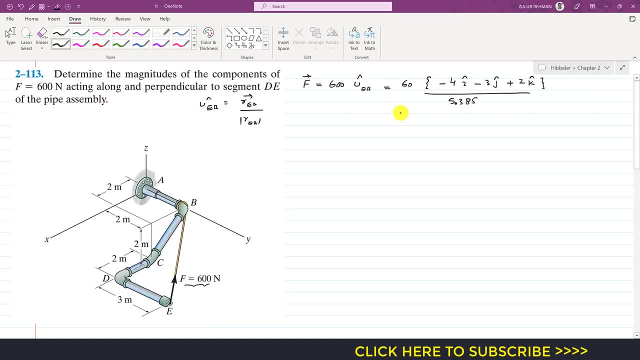 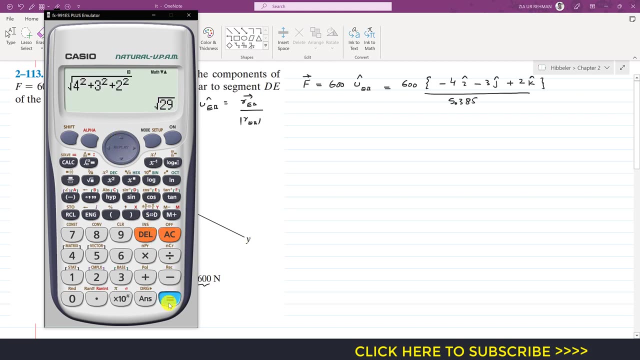 if i divide this 60 by its magnitude, so 60 divided by that answer, so this is 11.14. this, this is not 60, this is 600. so 600 divided by 600 divided by square root, 29, so this gives us 111.42, so 111.42. 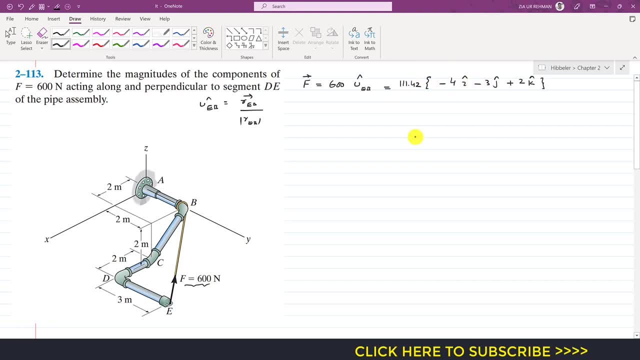 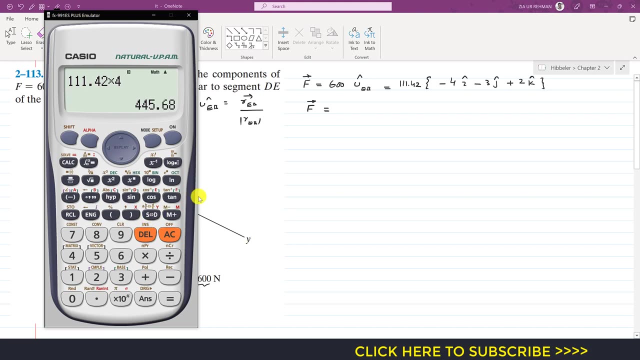 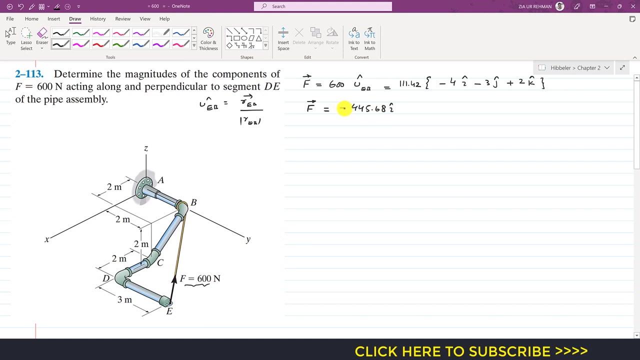 and now we will multiply this with, with each and every component, so we will get the cartesian vector representation of that force, f, which is acting from e to b. so 111.42 multiply by 4, so this is 445.68 i, and plus into minus is minus. again, plus into minus is minus. 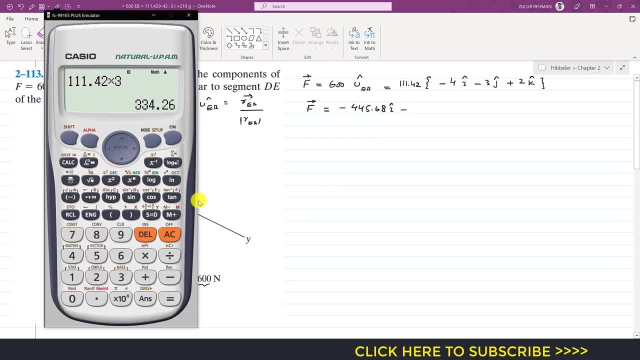 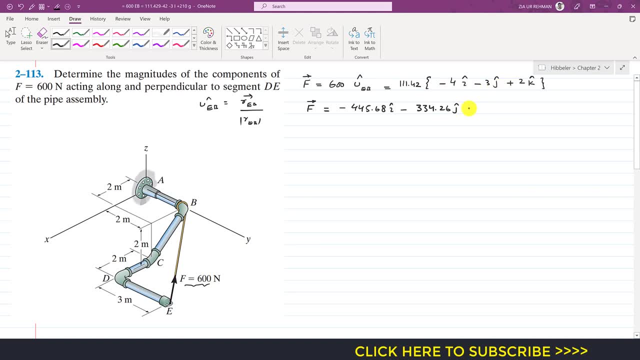 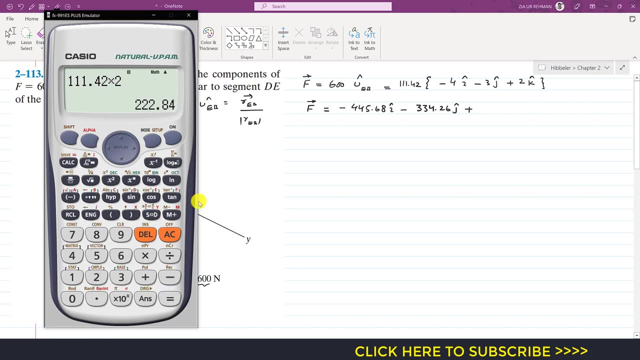 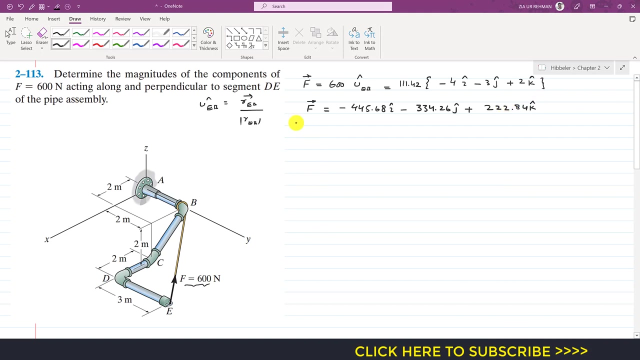 multiply by 334.26 j, and then multiply by 2, and plus into plus is plus. so multiply by 2, this is 222.84, 222.84 in the positive key. so this is the cartesian vector f which is acting from e to b. now we need to find the component of this force. 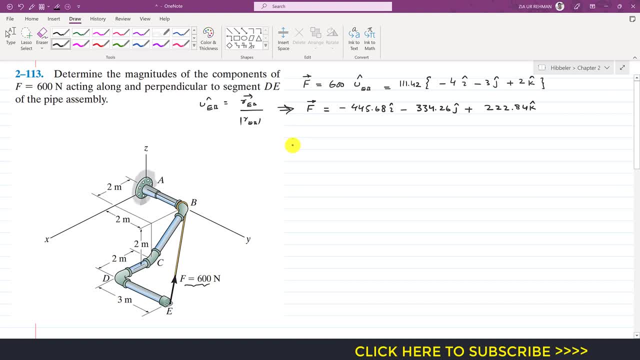 f along d e, which is parallel to it. right, so we can write that the component of force f along d e and which is parallel so we we need to determine its magnitude. so then that magnitude will be equal to the force f dot, the unit vector along d e. right, so we need to find the unit vector along which we. 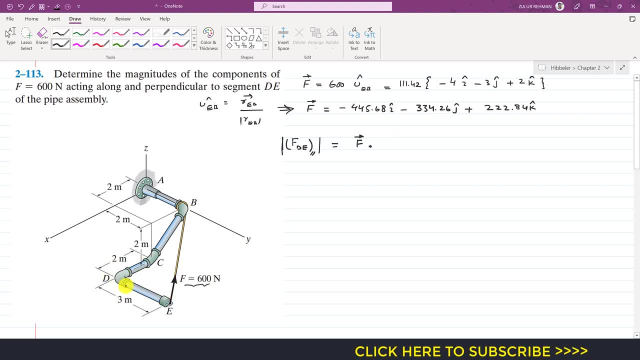 want to find the component right, so that d e we need to write the unit vector along d e, since we are interested to find the component of this force f along the d e, so i will multiply it with the unit vector along d e. so we know that force f. that force f is minus 445.68 i minus 334.26 j. 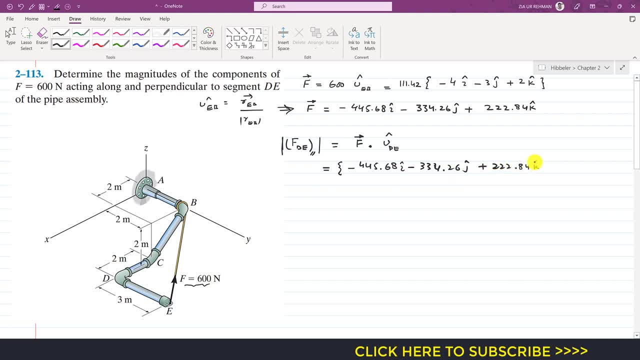 plus 222.84 k dot. and as we can see that this d e portion of the pipe is parallel to the y-axis, so this means that the unit vector along d e will be equal to the unit vector along y. so the unit vector along y is j, right, so the unit vector along d e is also j. 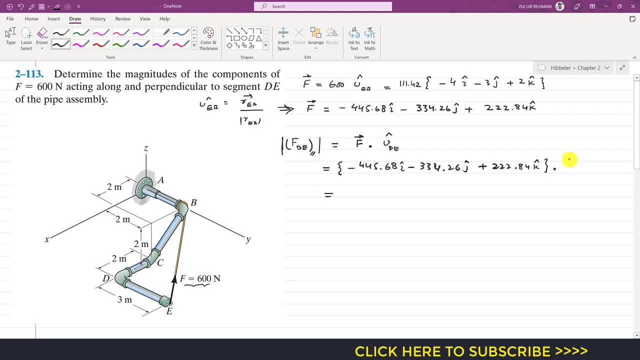 so this means that if we come, if we write complete unit vector along the j, so that will be equal to 0 i plus j plus 0 k. so now if we take the dot product, so i dot i, j, dot j and k dot k, so i. 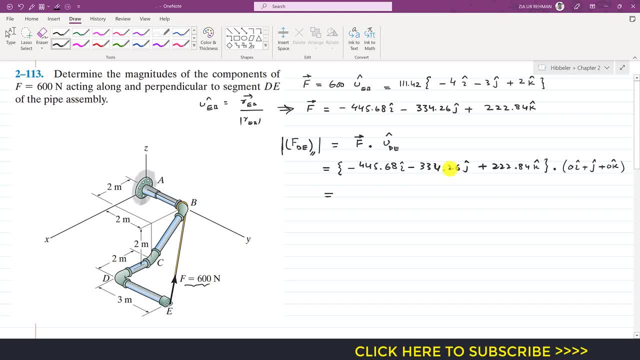 dot i is 0. this into 0 is 0, so only the j term will. we will be left with the j term right and j dot j is 1.. so we will be left with minus 334.26 into 1. we can say: multiply by 1 and j dot j, so j dot j is 1 and we will get. 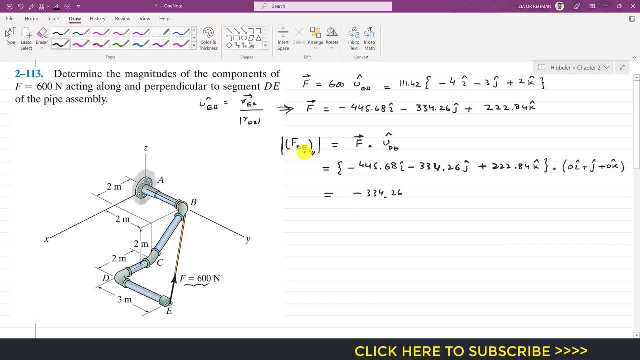 minus 334.26 as the magnitude of the component of d e which is parallel to that d e portion of the pipe, and this is in newton. now the negative science tells us that the component of that force, f, along d e, has an opposite sense of direction, that is, to u d e that the 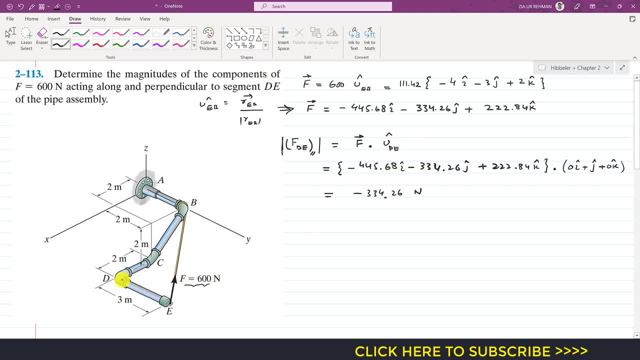 position vector along d e is in in this direction, but the component which is parallel to the d e of that force f is acting in this direction. so the negative sign tells us the sense of the direction right. so this is the component of d e which is parallel to that d e portion of the pipe. now 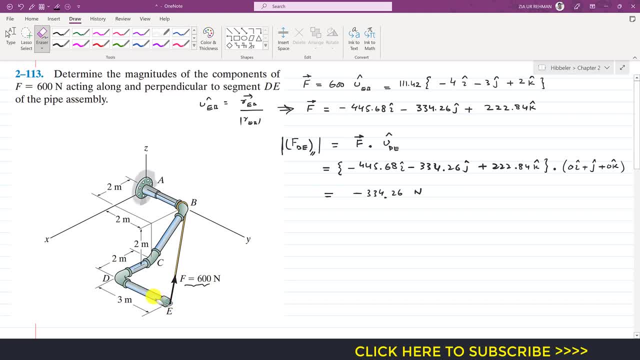 if i draw that component, so that component of the force along d e is acting like this, and then the perpendicular component of that force, f, which will be perpendicular to this d e. so if i represent that, so let's say that this component is f, d e perpendicular and let's say that it is making